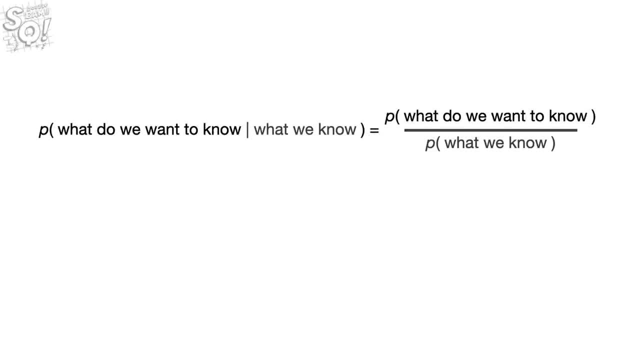 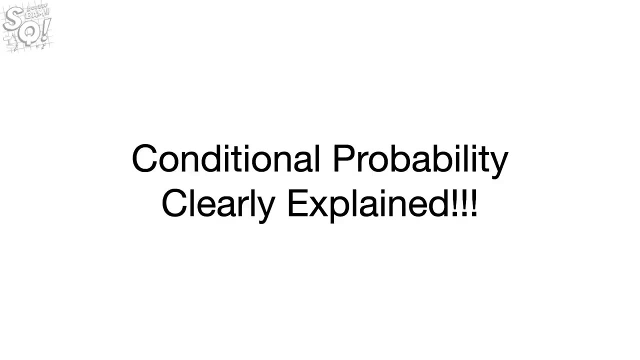 What do we want to know, Scaled by what we know- StatQuest. Hello, I'm Josh Darmer and welcome to StatQuest. Today we're going to talk about conditional probability, and it's going to be clearly explained. First, let's go to the magical place called StatLand. 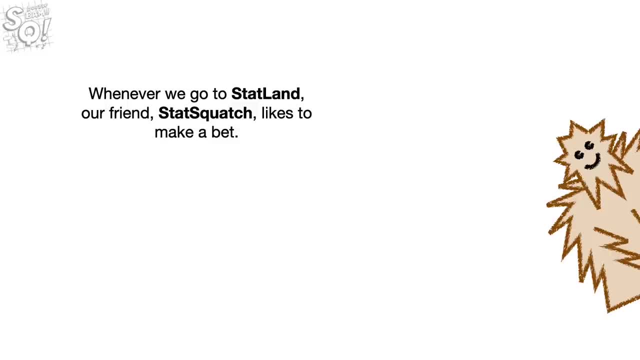 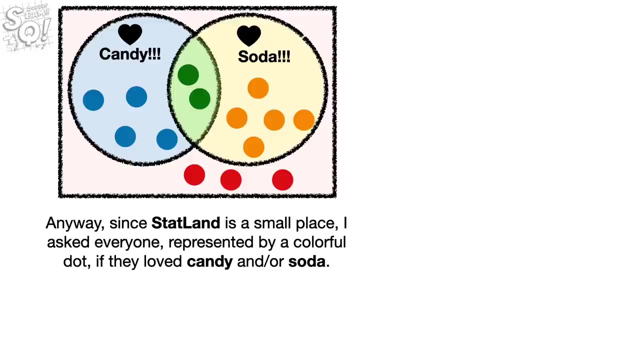 Whenever we go to StatLand, our friend Statsquatch likes to make a bet. I bet you $1 that the next person we meet loves candy and soda. Anyway, since StatLand is a small place, I asked everyone, represented by a colorful dot, if they loved candy and or soda. 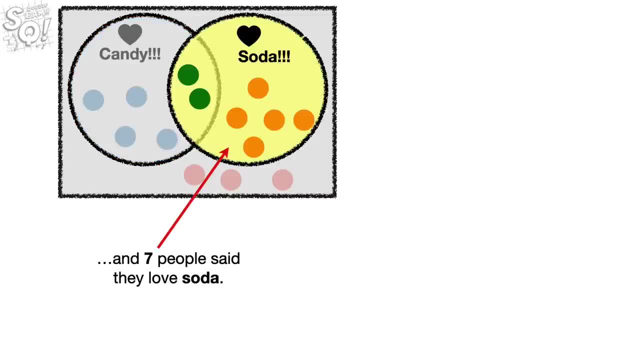 Six people said they love candy And seven people said they love soda. And of the people that loved candy or soda, two people said they loved both. So let's go to StatLand. And last but not least, three people in StatLand said they did not love candy or soda. 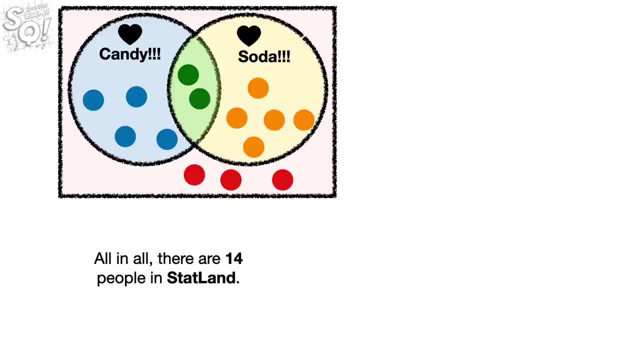 All in all, there are 14 people in StatLand. One way to keep track of this data is to put it into something called a contingency table. In this case, the rows are for keeping track of people that love soda or do not love soda. 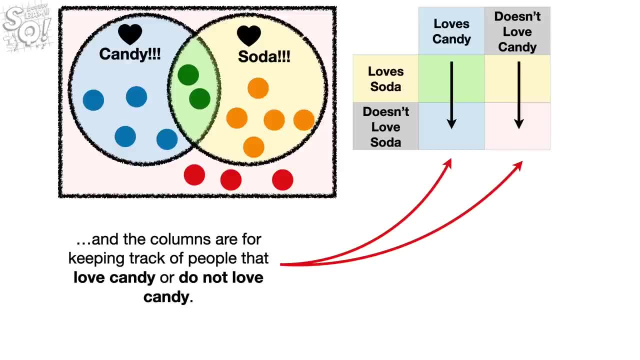 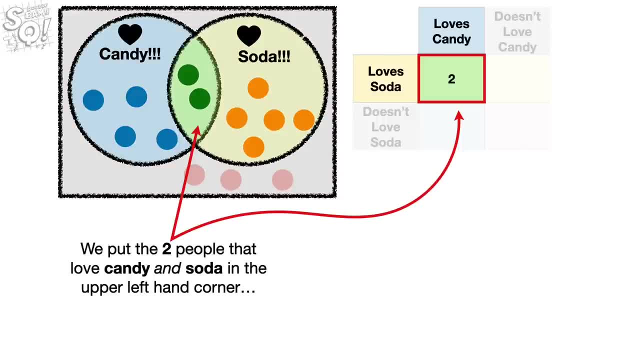 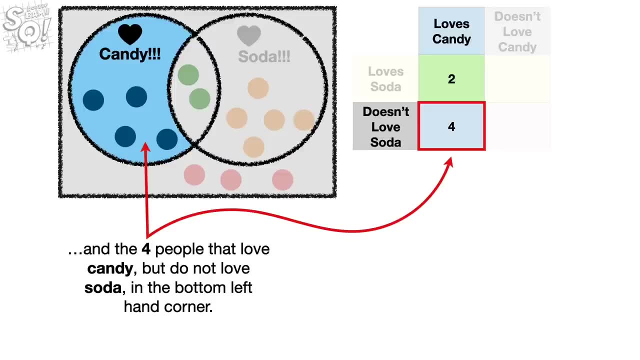 And the columns are for keeping track of people that love candy or do not love candy. We put the two people that love candy and soda in the upper left-hand corner And the four people that love candy but do not love soda in the bottom left-hand corner. 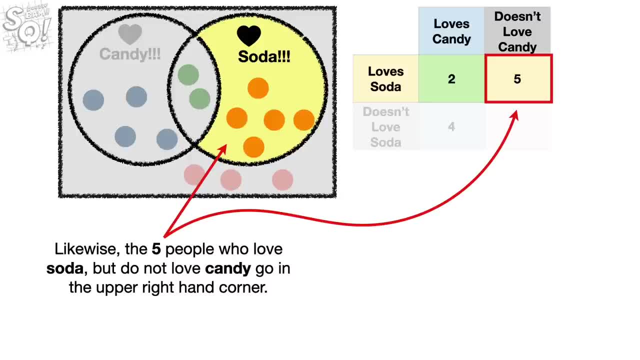 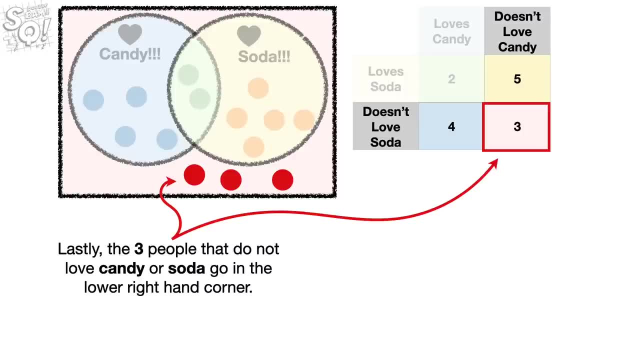 Likewise, the five people who love soda but do not love candy go in the upper right-hand corner. Lastly, the three people that do not love candy or soda go in the lower right-hand corner. So we can use this data to calculate the number of people that love candy and soda. 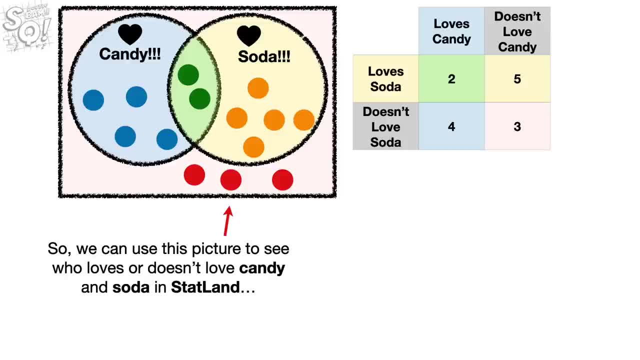 We can use this picture to see who loves or doesn't love candy and soda in StatLand. Or we can use this contingency table. They both contain the same information. Bam, Now, remember the bet our friend Statsquatch wanted to make. 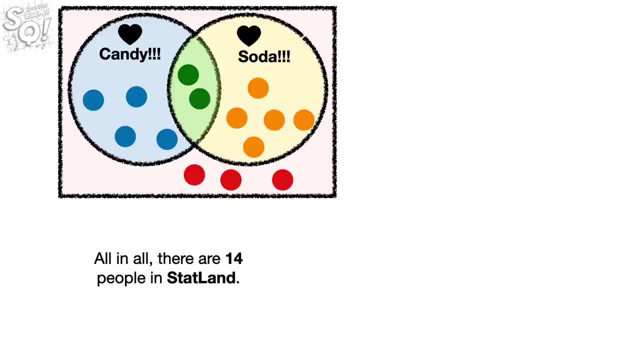 All in all, there are 14 people in StatLand. One way to keep track of this data is to put it into something called a contingency table. In this case, the rows are for keeping track of people that love soda or do not love soda. 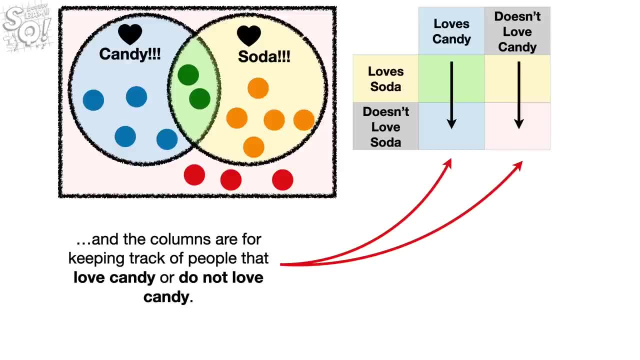 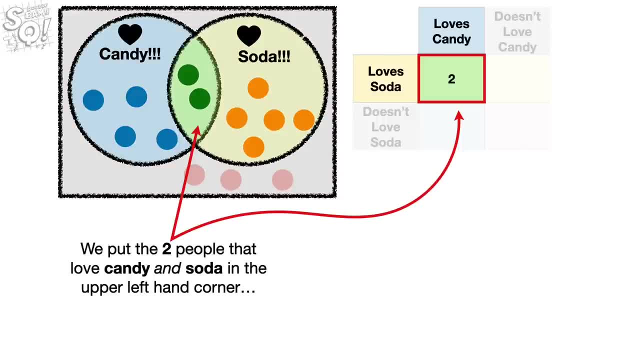 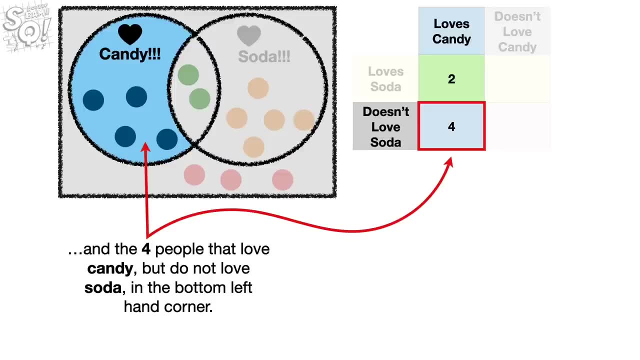 And the columns are for keeping track of people that love candy or do not love candy. We put the two people that love candy and soda in the upper left-hand corner And the four people that love candy but do not love soda in the bottom left-hand corner. 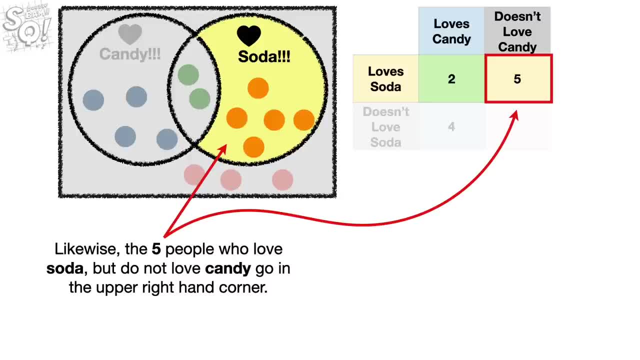 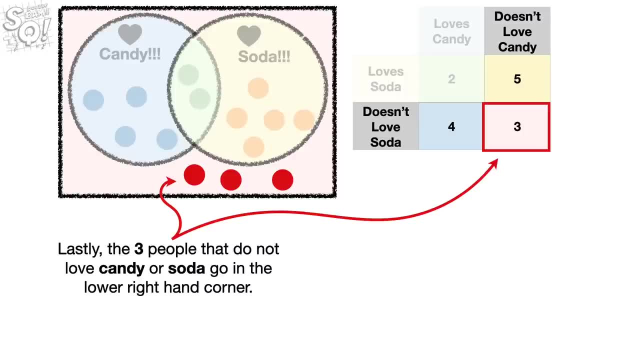 Likewise, the five people who love soda but do not love candy go in the upper right-hand corner. Lastly, the three people that do not love candy or soda go in the lower right-hand corner. So we can use this data to calculate the number of people that love candy and soda. 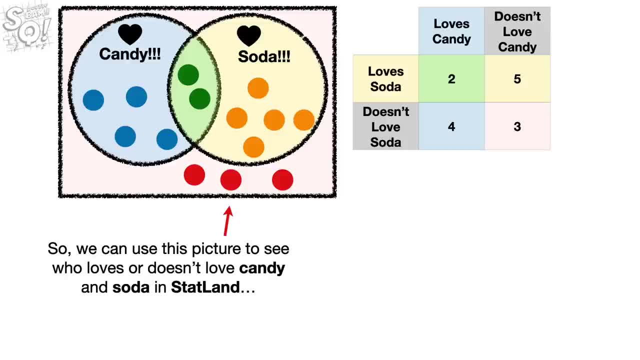 We can use this picture to see who loves or doesn't love candy and soda in StatLand. Or we can use this contingency table. They both contain the same information. Bam, Now, remember the bet our friend Statsquatch wanted to make. 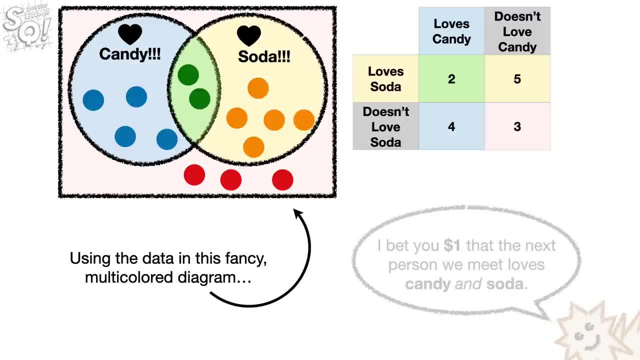 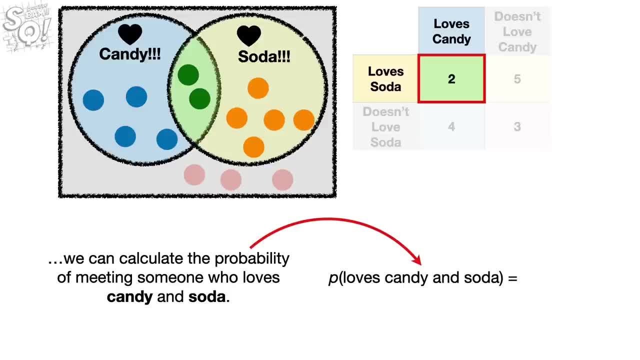 Using the data in this fancy multicolored diagram or this crazy technicolor table, we can calculate the probability of meeting someone who loves candy and soda. The P in this fancy statistics notation is short for probability, So this whole thing says the probability that someone loves candy and soda. 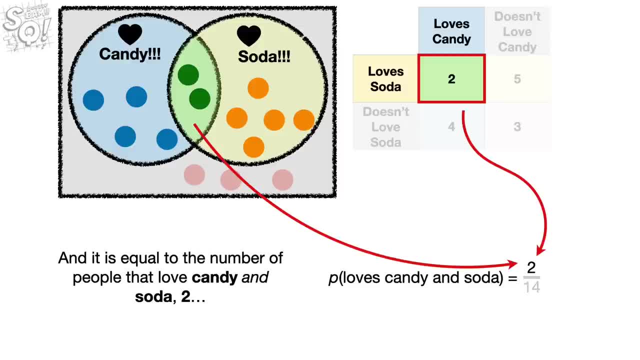 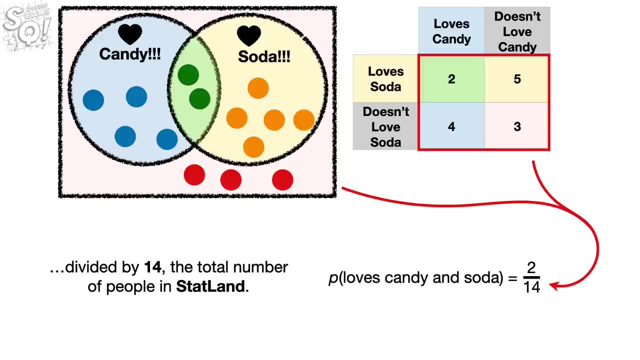 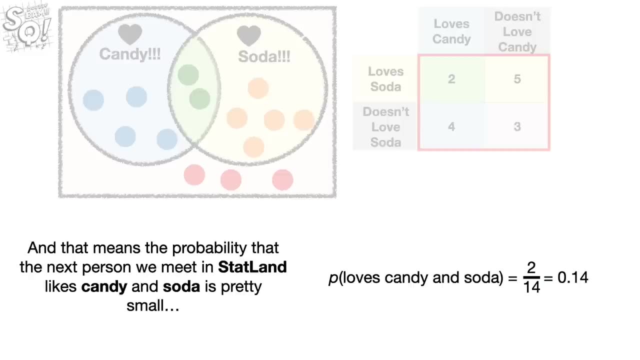 And it is equal to the number of people that love candy and soda too- divided by 14, the total number of people in StatLand, And when we do the math, we get 0.14.. And that means the probability that the next number of people in StatLand will give us 0.14. 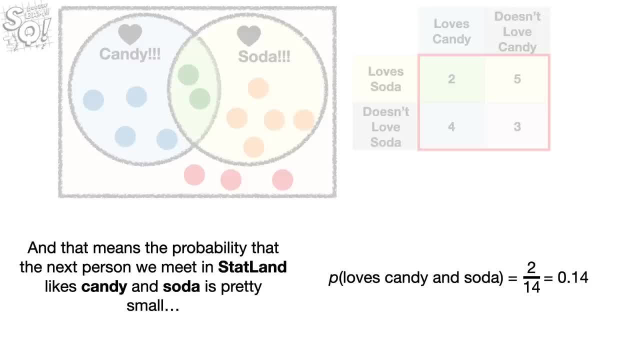 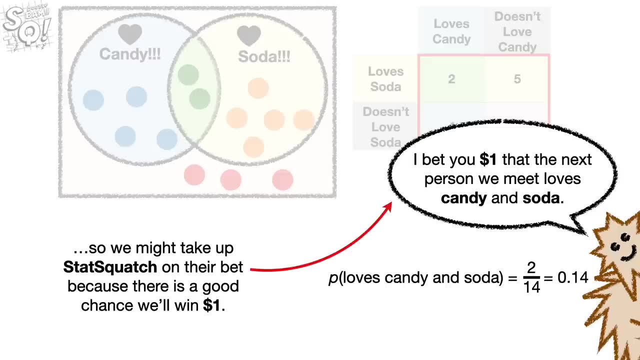 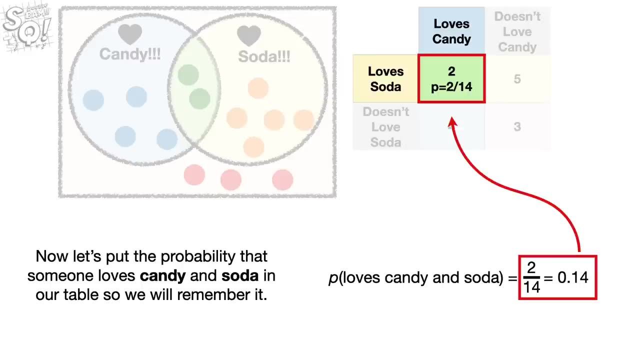 person we meet in StatLand likes candy and soda is pretty small, So we might take up StatSquatch on their bet, because there's a good chance we'll win one dollar Bam. Now let's put the probability that someone loves candy and soda in our 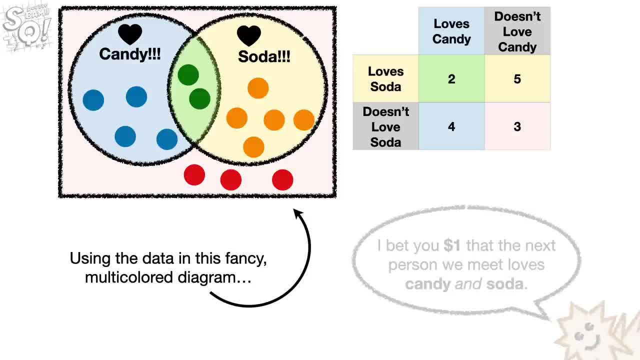 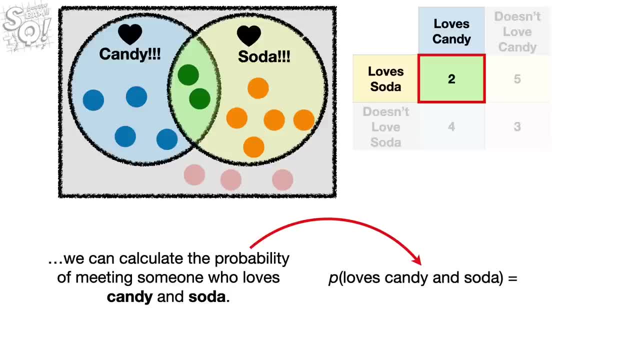 Using the data in this fancy multicolored diagram or this crazy technicolor table, we can calculate the probability of meeting someone who loves candy and soda. The P in this fancy statistics notation is short for probability, So this whole thing says the probability that someone loves candy and soda. 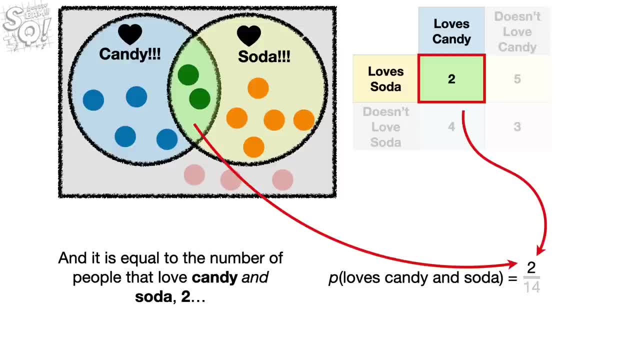 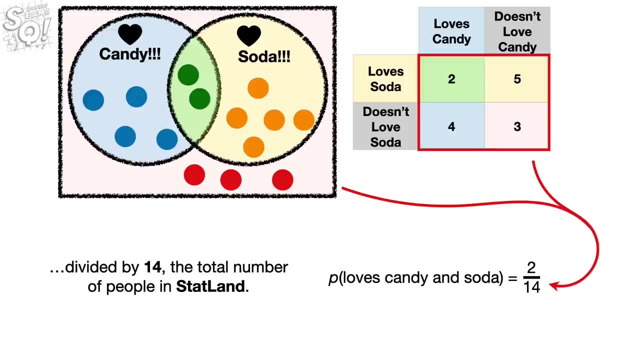 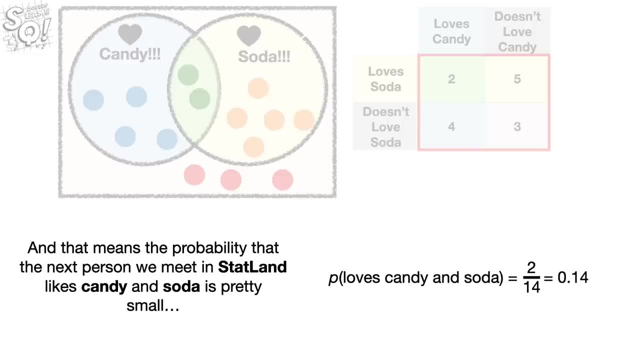 And it is equal to the number of people that love candy and soda. two divided by 14, the total number of people in StatLand, And when we do the math we get 0.14.. And that means the probability that. 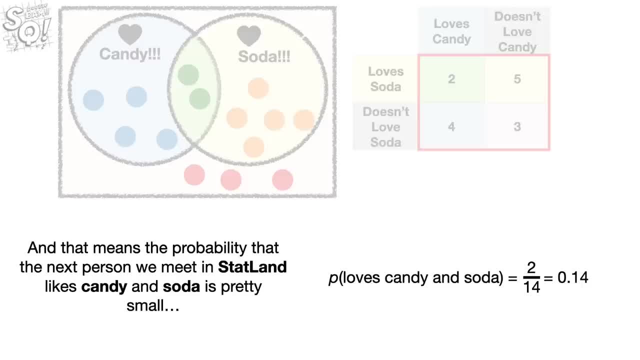 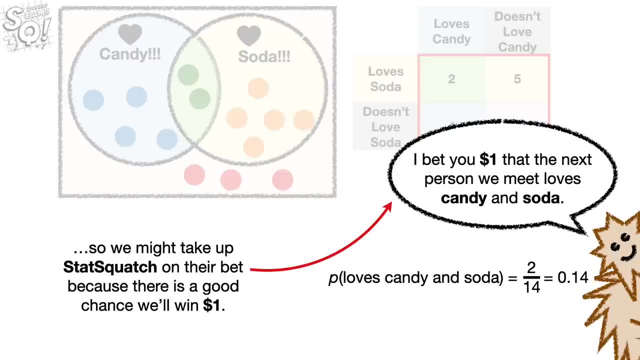 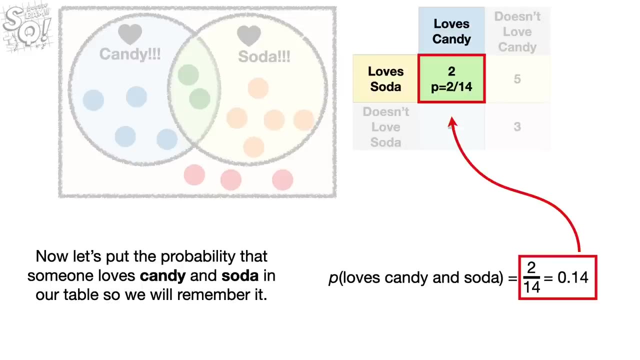 the next friend loves candy and soda is four person we meet in StatLand likes candy and soda is pretty small, So we might take up StatSquatch on their bet, because there's a good chance we'll win one dollar. Bam. Now let's put the probability that someone loves candy and soda in our 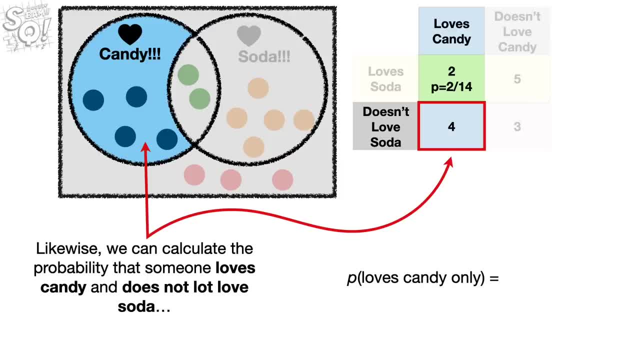 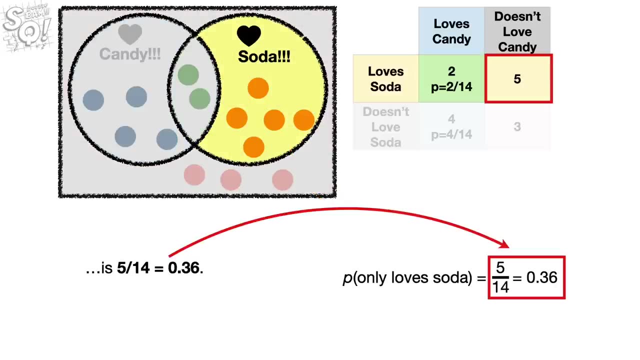 table, so we will remember it. Likewise, we can calculate the probability that someone loves candy and does not love soda, and we get 0.29.. The probability that someone loves soda but not candy is 5 divided by 14, which equals 0.36, and the 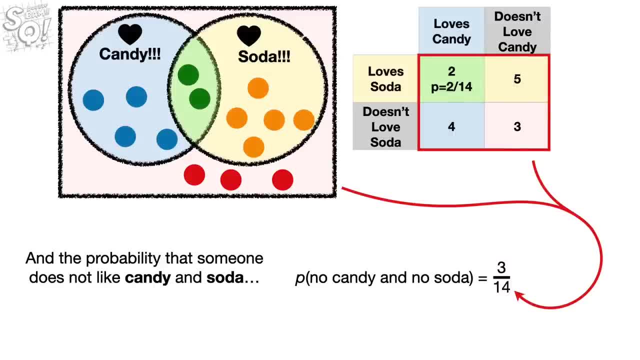 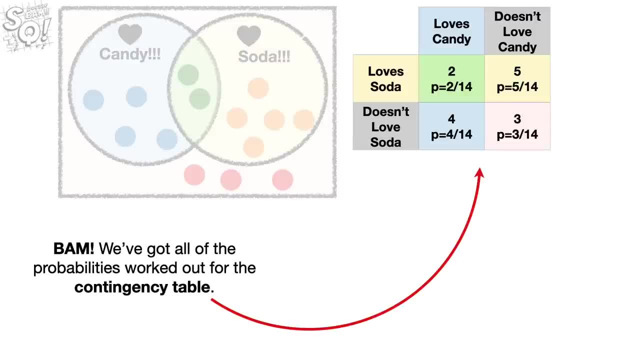 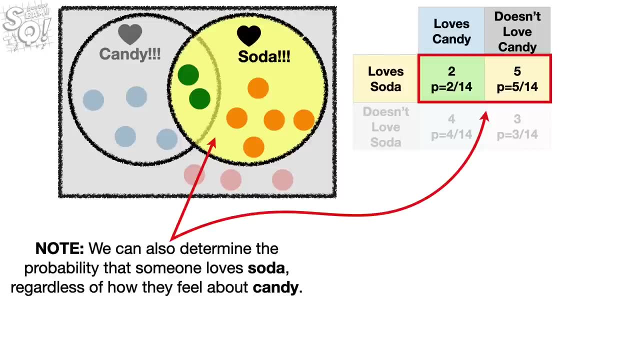 probability that someone does not like candy and soda is 3 divided by 14, which equals 0.21.. Bam, We've got all of the probabilities already worked out for the contingency table. Note: we can also determine the probability that someone loves soda regardless of how. 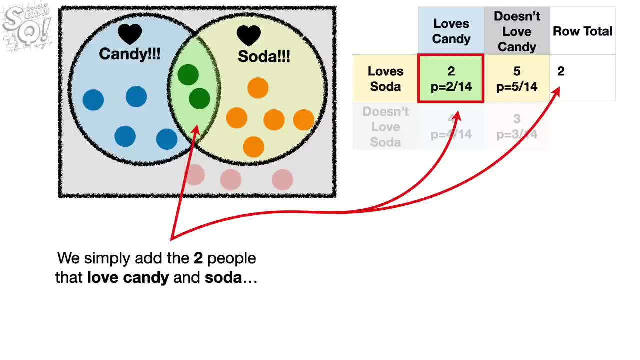 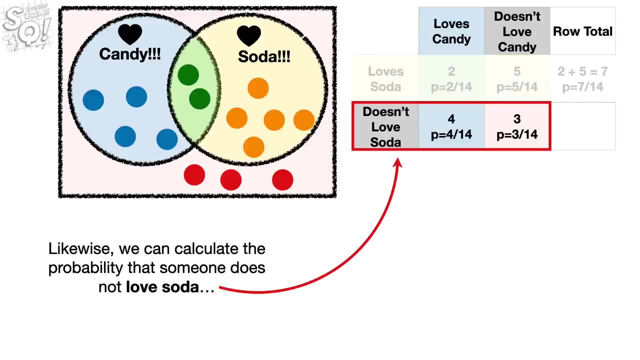 they feel about candy. We simply add the two people that love candy and soda to the five people that love soda but not candy and divide that sum by 14, the population of StatLand. Likewise, we can calculate the probability that someone does not love soda by adding up. 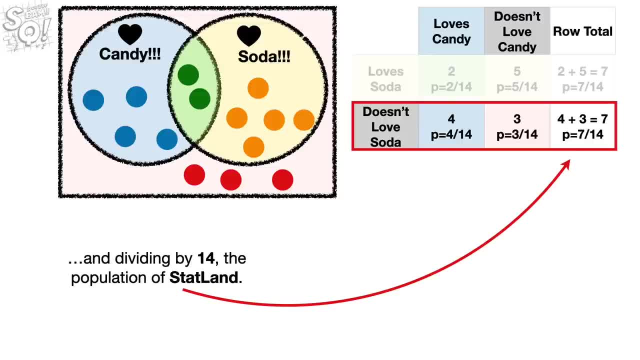 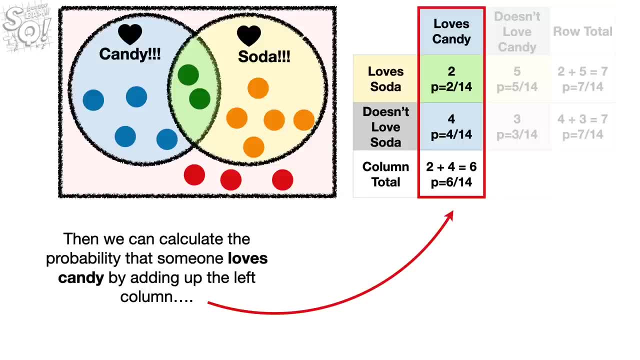 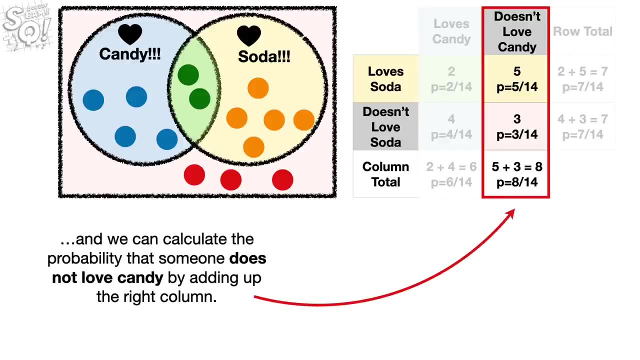 the counts in the bottom row and dividing by 14, the population of StatLand, Then we can calculate the probability that someone loves candy by adding up the left column And we can calculate the probability that someone does not love candy by adding up the right column. 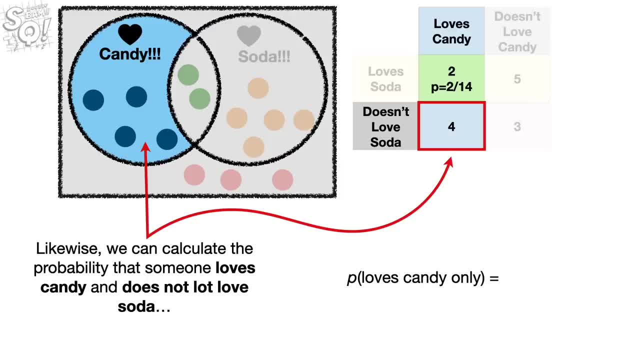 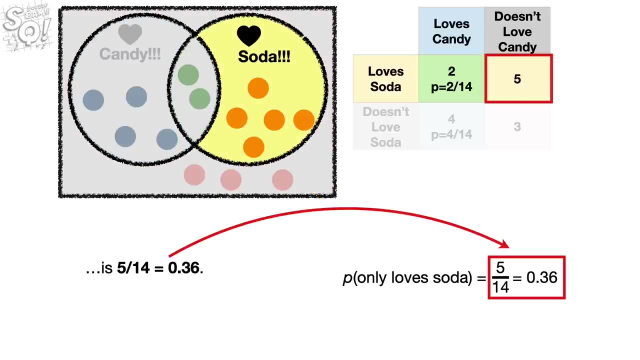 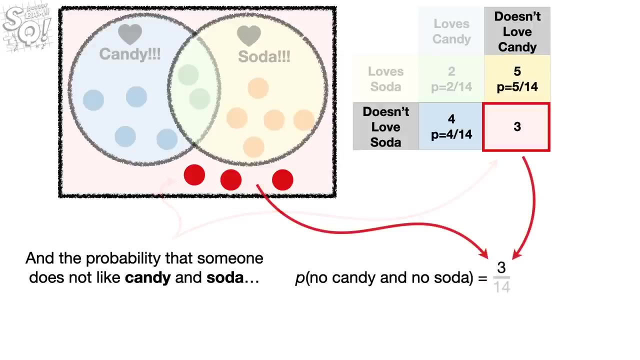 table, so we will remember it. Likewise, we can calculate the probability that someone loves candy and does not love soda, and we get 0.29.. The probability that someone loves soda but not candy is 5 divided by 14, which equals 0.36,, and the probability that someone does not like candy and soda is: 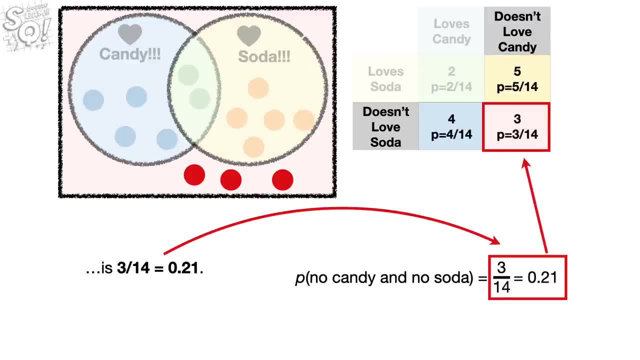 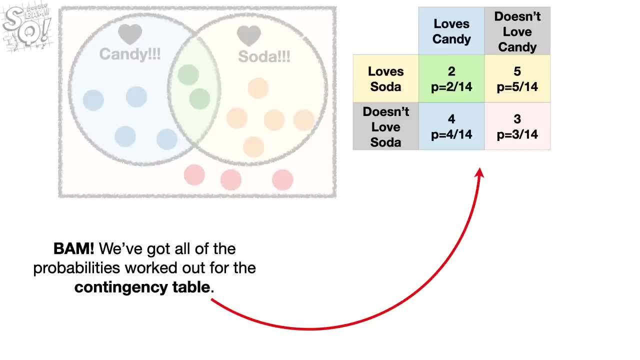 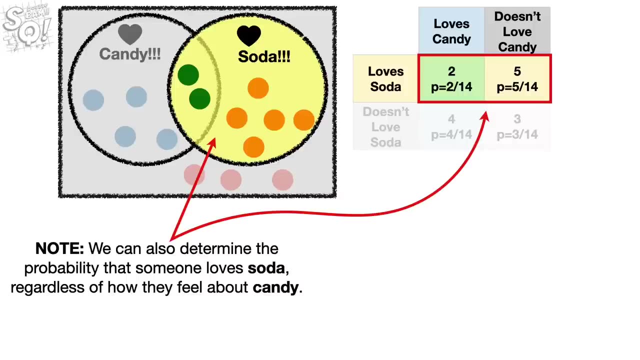 3 divided by 14, which equals 0.21.. Bam, We've got all of the probabilities already worked out for the contingency table. Note: we can also determine the probability that someone loves soda regardless of how they feel about candy. 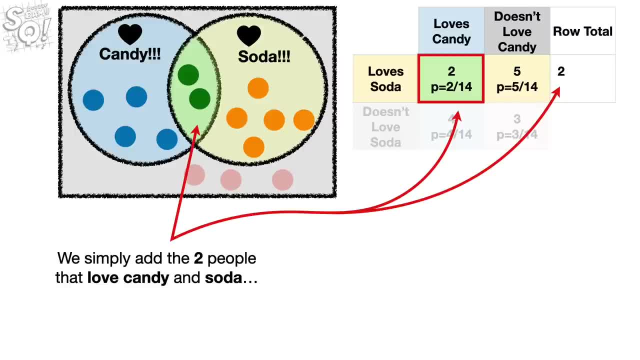 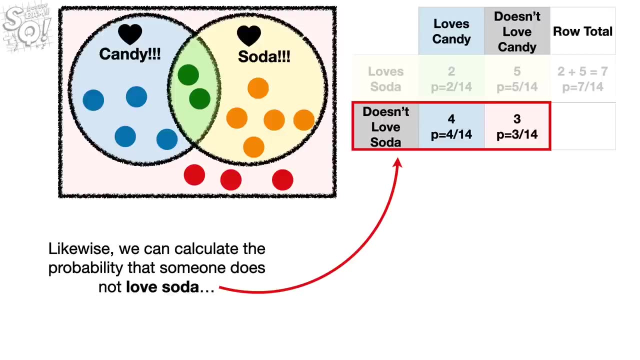 We simply add the two people that love candy and soda to the five people that love soda but not candy and divide that sum by 14, the population of StatLand. Likewise, we can calculate the probability that someone does not love soda by adding up: 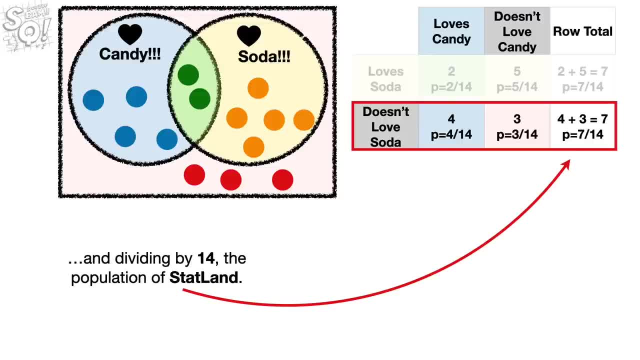 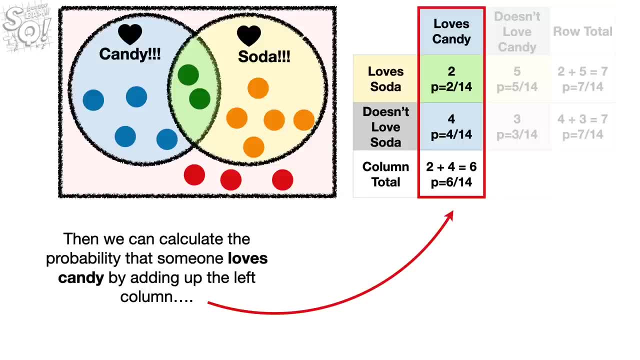 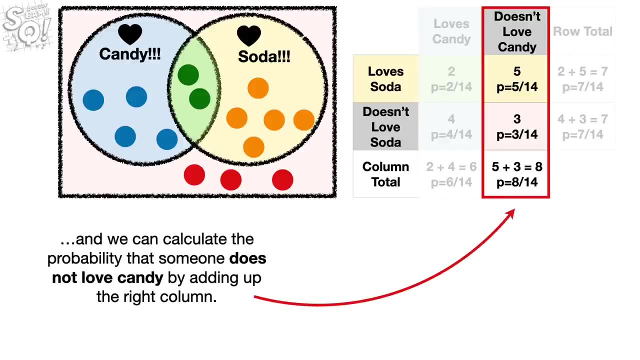 the counts in the bottom row and dividing by 14, the population of StatLand, Then we can calculate the probability that someone loves candy by adding up the left column And we can calculate the probability that someone does not love candy by adding up the right column. 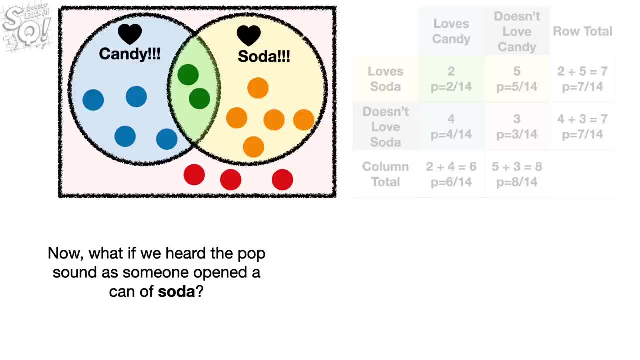 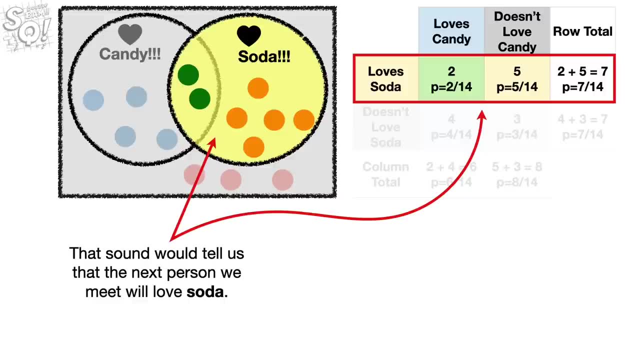 Bam. Now what if we heard the pop sound as someone opened a can of soda? That sound would tell us that the next person we meet will love soda. Knowing that the next person we meet will love soda, what is the probability that the next person also loves candy? 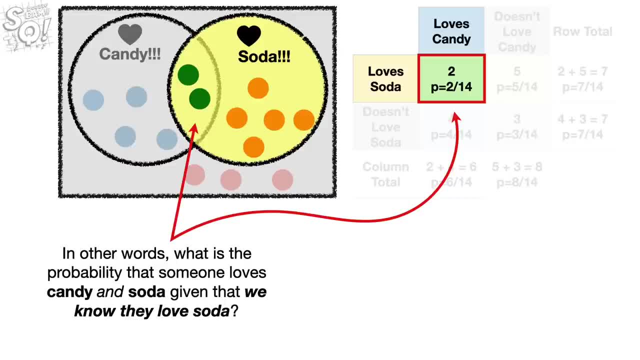 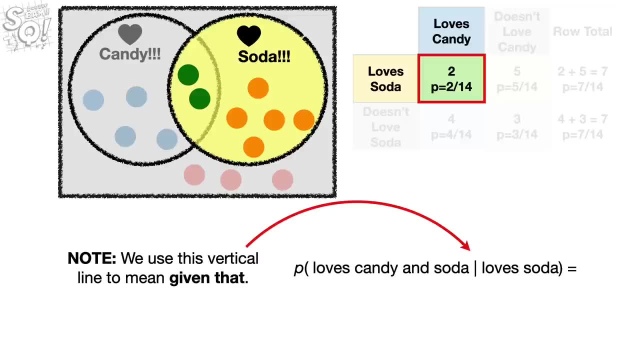 In other words, what is the probability that someone loves candy and soda, given that we know they love soda? Note, we use this vertical line to mean given that. So this is the probability that the next person we meet loves candy and soda, given that we know they love soda. 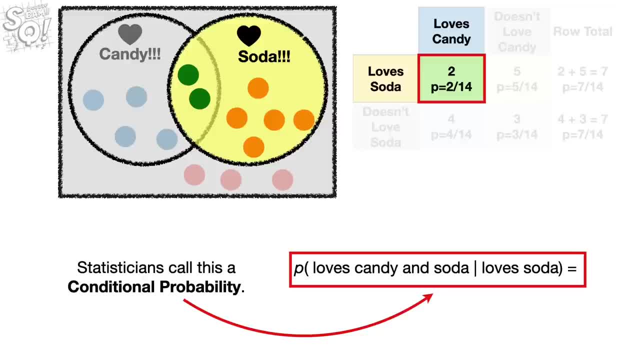 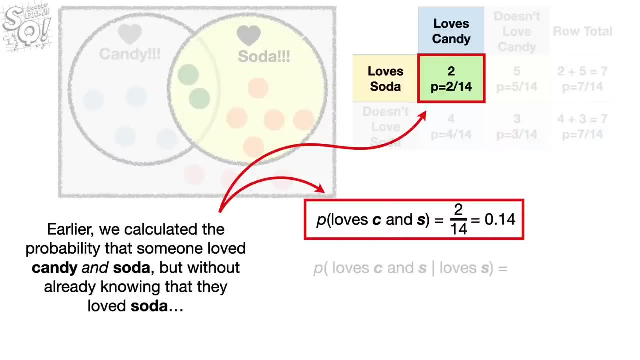 Statisticians call this a conditional probability. Bam Note, I hate using abbreviations, but let's let candy equal C and soda equal S. Earlier we calculated the probability that someone loved candy and soda, but without already knowing that they loved soda. 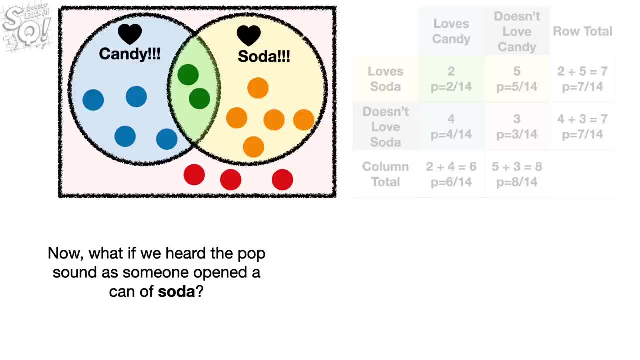 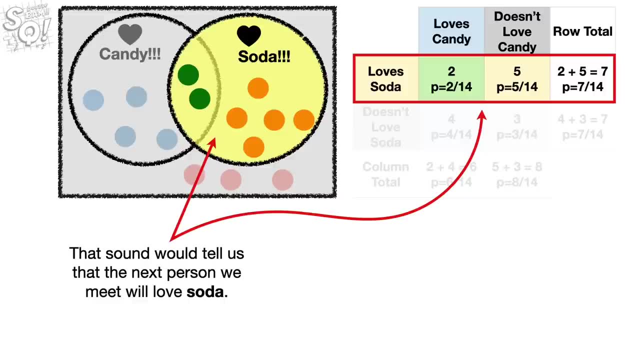 Bam. Now what if we heard the pop sound as someone opened a can of soda? That sound would tell us that the next person we meet will love soda. Knowing that the next person we meet will love soda, what is the probability that the next person also loves candy? 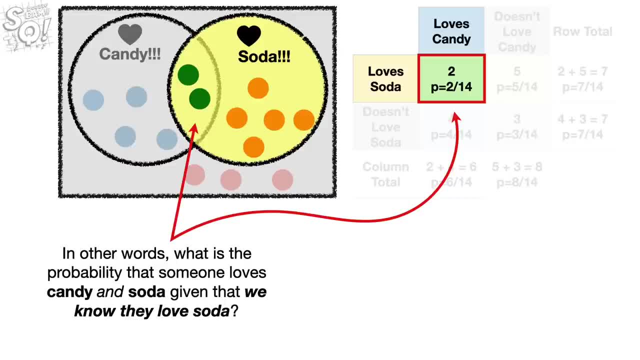 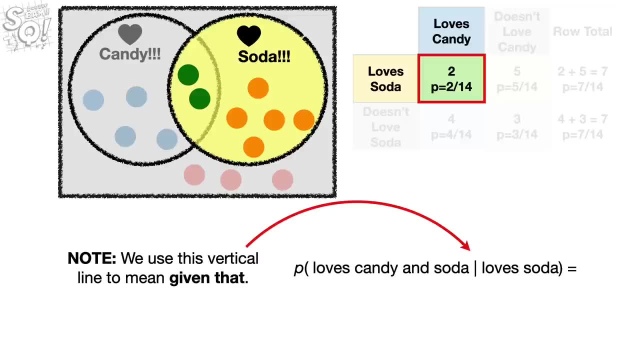 In other words, what is the probability that someone loves candy and soda, given that we know they love soda? Note, we use this vertical line to mean given that. So this is the probability that the next person we meet loves candy and soda, given that we know they love soda. 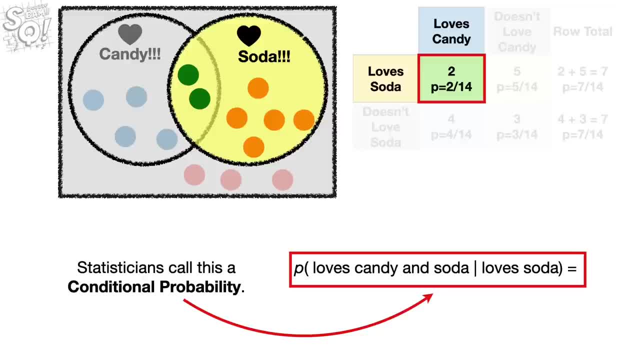 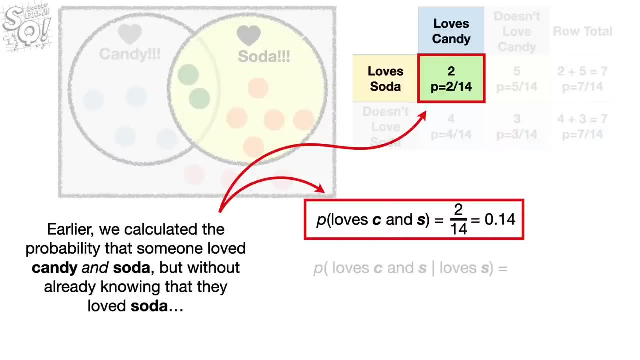 Statisticians call this a conditional probability. Bam Note, I hate using abbreviations, but let's let candy equal C and soda equal S. Earlier we calculated the probability that someone loved candy and soda, but without already knowing that they loved soda. 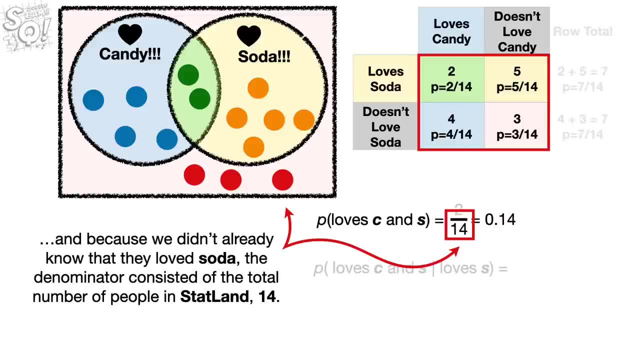 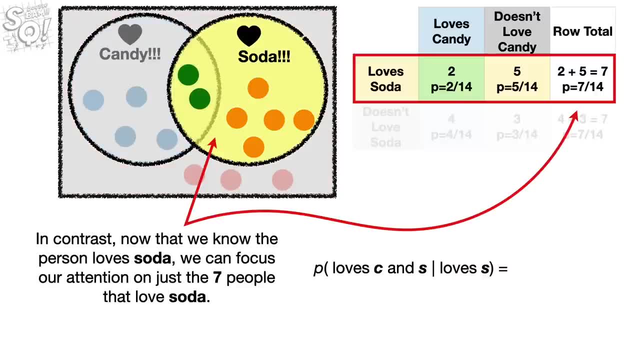 And because we didn't already know that they loved soda. the denominator consisted of the total number of people in StatLand 14.. In contrast, now that we know the person loves soda, we can focus our attention on just the seven people that love soda. 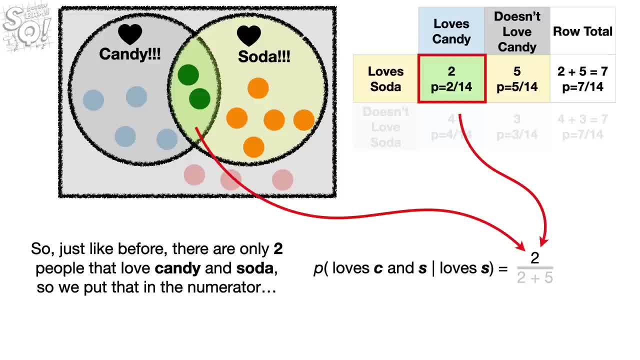 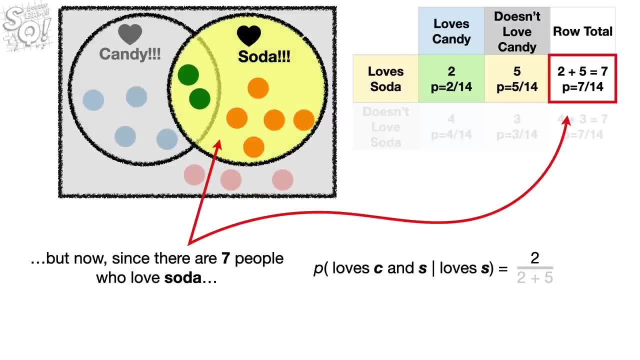 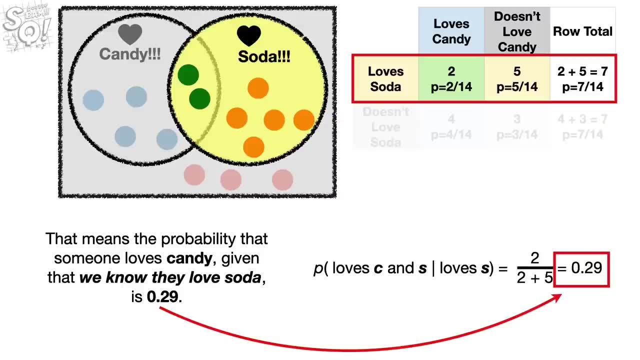 So, just like before, there are only two people that love candy and soda, so we put that in the numerator. But now, since there are seven people who love soda, we put that in the denominator. That means the probability that someone loves candy. 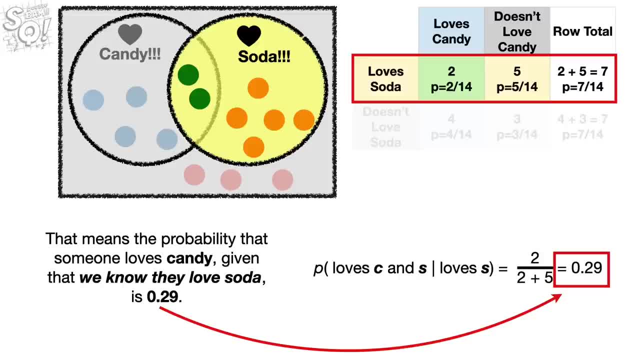 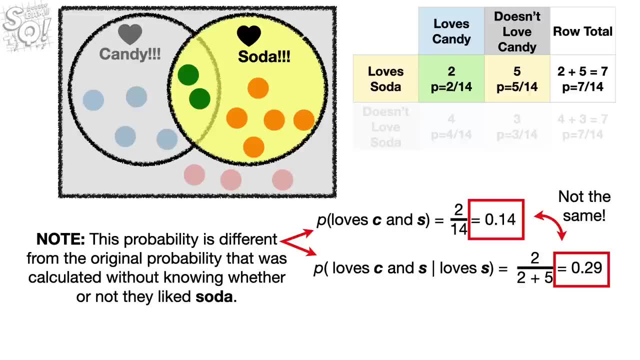 given that we know they love soda, is 0.29.. Note: this probability is different from the original probability that was calculated without knowing whether or not they like soda. In this case, knowing that they love soda increased the probability that they would love candy. 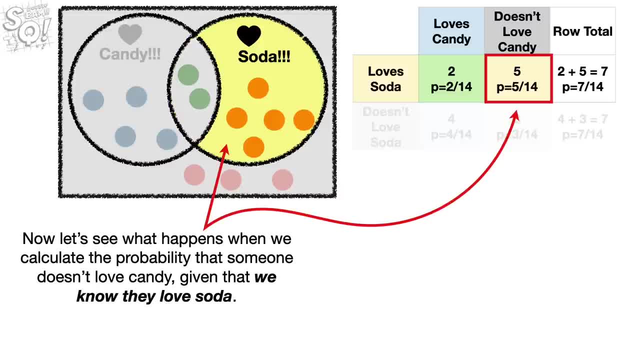 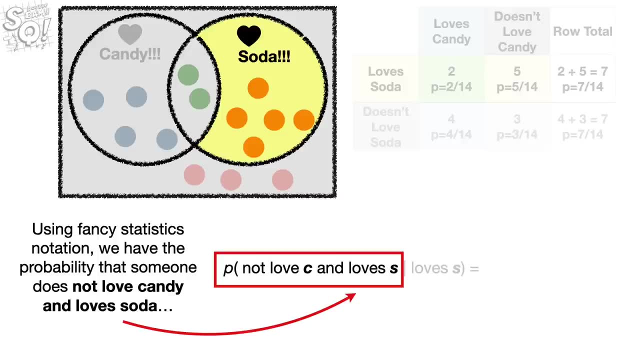 Duh, Double-bam. Now let's see what happens when we calculate the probability that someone doesn't love candy, given that we know they love soda. Using fancy statistics notation, we have the probability that someone does not love candy and loves soda, given that we know they love soda. 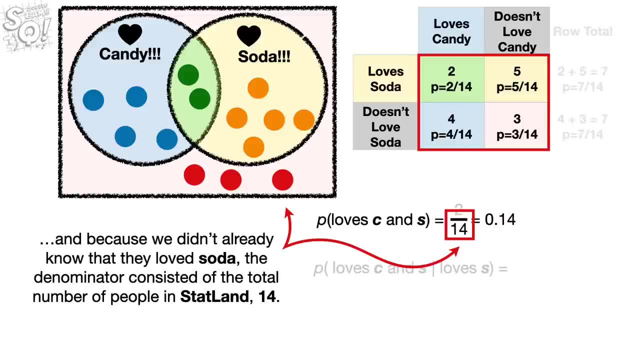 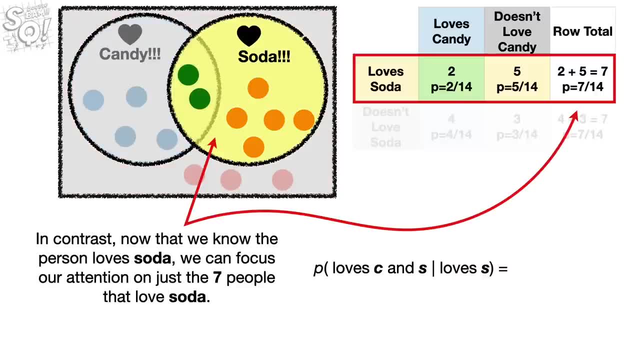 And because we didn't already know that they loved soda. the denominator consisted of the total number of people in StatLand 14.. In contrast, now that we know the person loves soda, we can focus our attention on just the seven people that love soda. 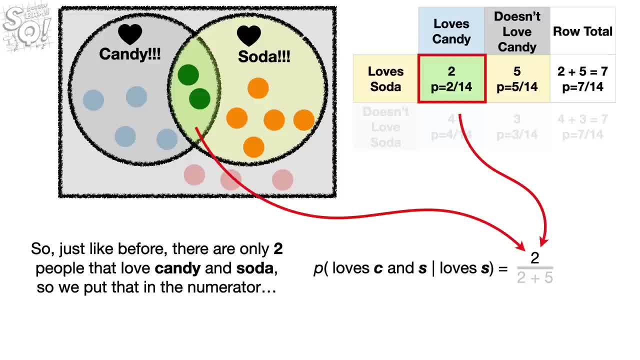 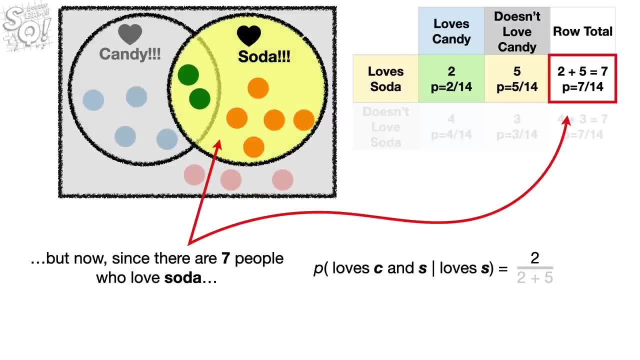 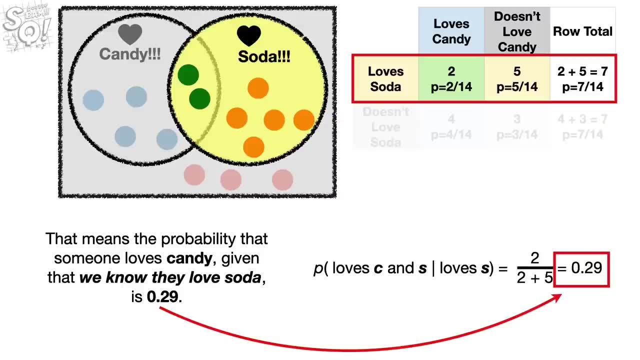 So, just like before, there are only two people that love candy and soda, so we put that in the numerator. But now, since there are seven people who love soda, we put that in the denominator. That means the probability that someone loves candy. 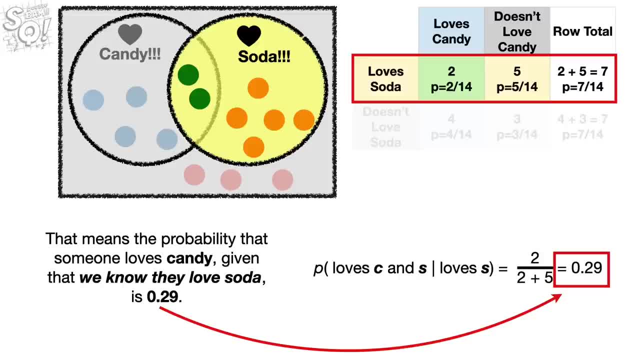 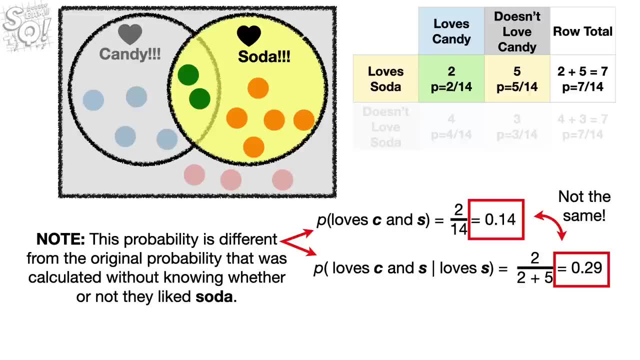 given that we know they love soda, is 0.29.. Note: this probability is different from the original probability that was calculated without knowing whether or not they like soda. In this case, knowing that they love soda increased the probability that they would love candy. 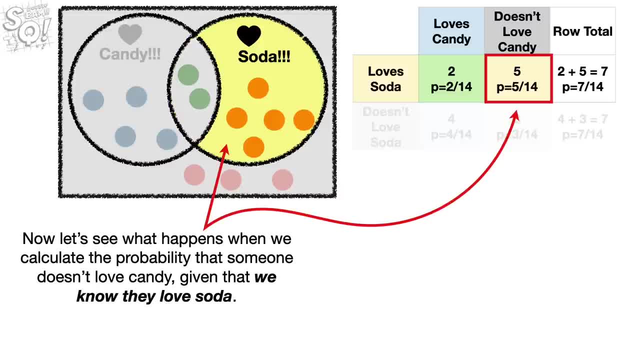 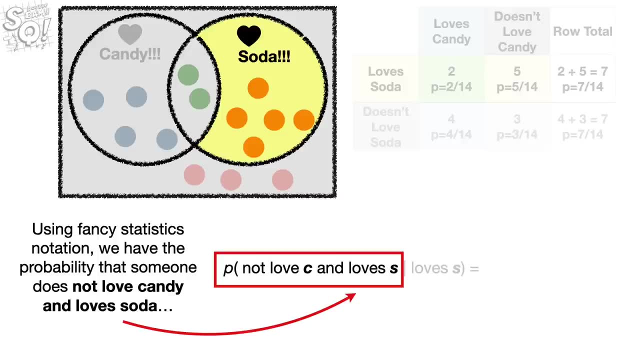 Duh, Double-bam. Now let's see what happens when we calculate the probability that someone doesn't love candy, given that we know they love soda. Using fancy statistics notation, we have the probability that someone does not love candy and loves soda, given that we know they love soda. 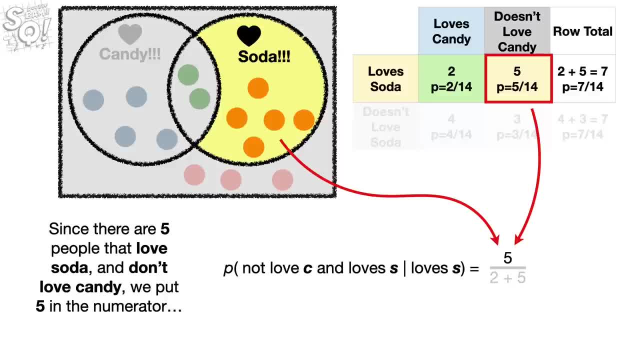 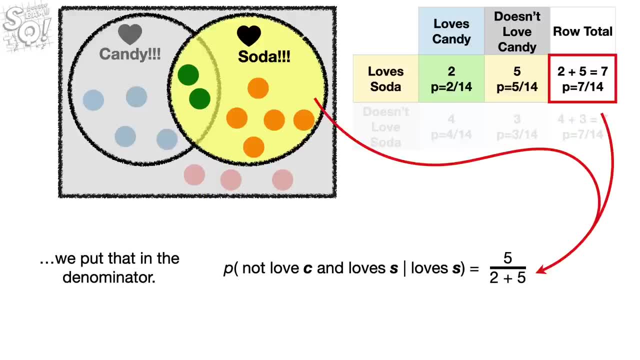 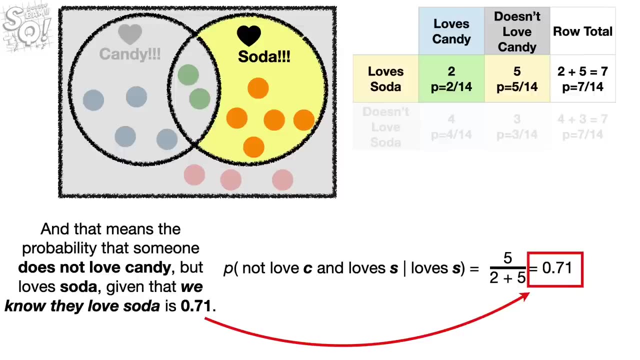 Since there are five people that love soda and don't love candy, we put five in the numerator, And since there are seven people who love soda, we put that in the denominator, And that means the probability that someone does not love candy but loves soda, given that we know, 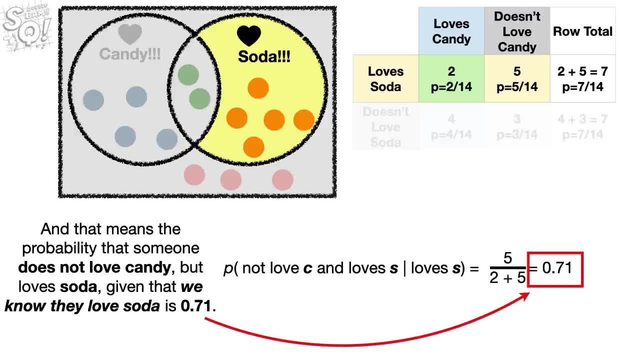 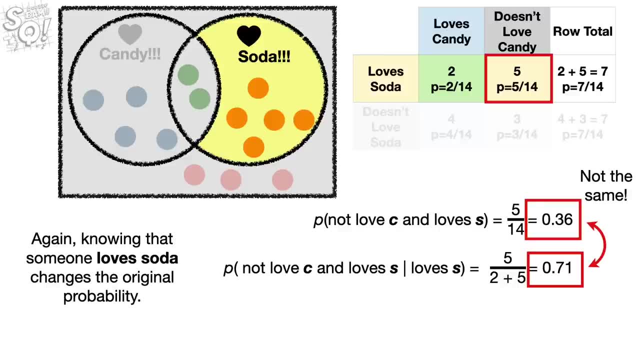 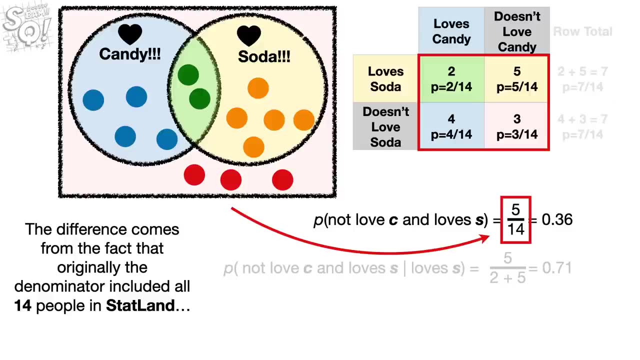 they love soda is 0.71.. Again, knowing that someone loves soda changes the original probability. The difference comes from the fact that originally the denominator included all the other variables. It included all 14 people in StatLand, But once we know they love soda. 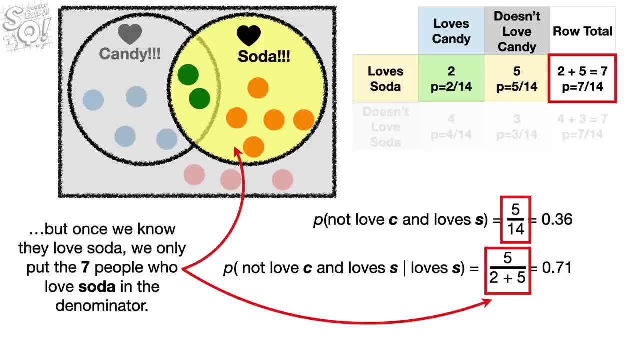 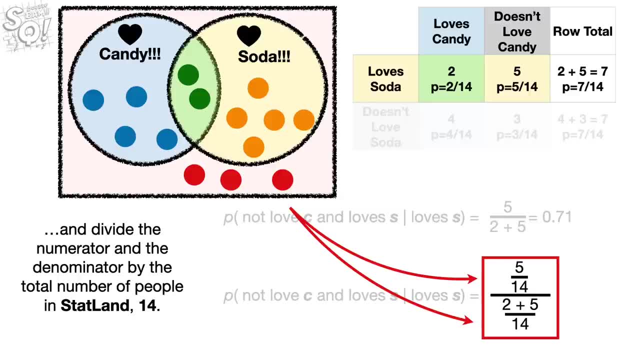 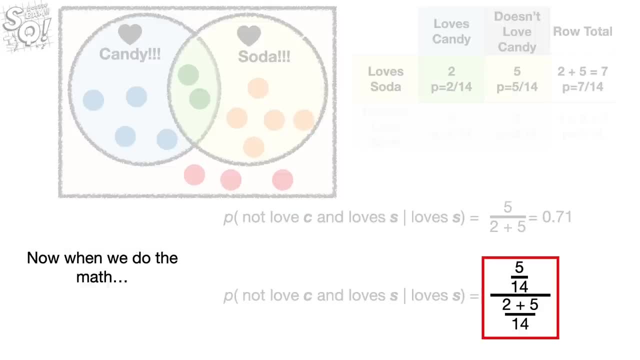 we only put the seven people who love soda in the denominator. Now let's make a copy of the conditional probability and divide the numerator and the denominator by the total number of people in StatLand 14.. Now when we do the math, we get 0.71,. 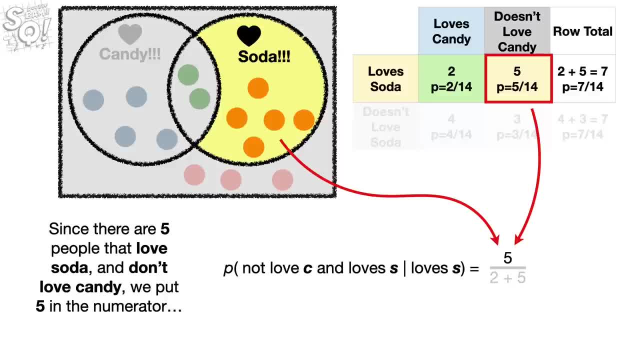 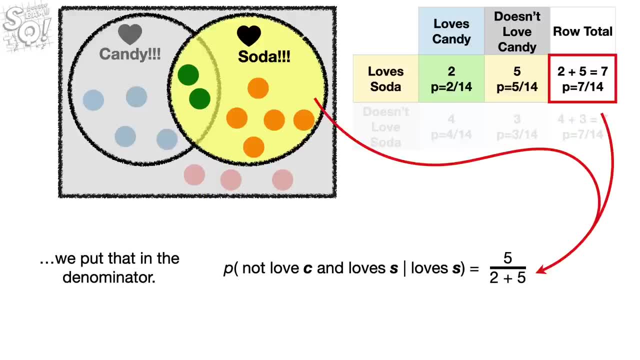 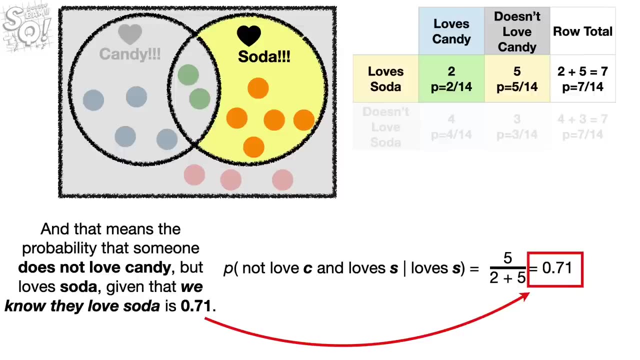 Since there are five people that love soda and don't love candy, we put five in the numerator, And since there are seven people who love soda, we put that in the denominator, And that means the probability that someone does not love candy but loves soda, given that we know, 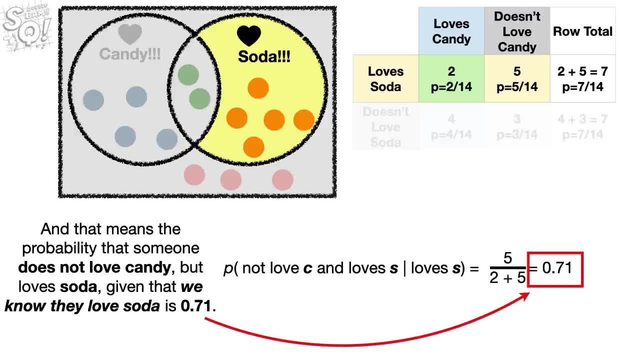 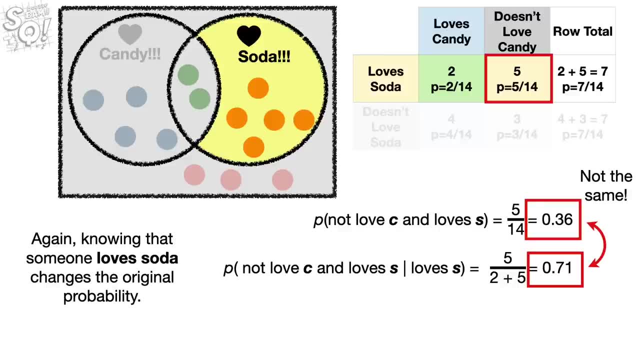 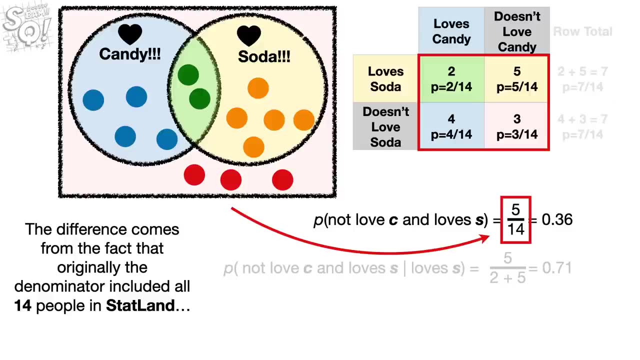 they love soda is 0.71.. Again, knowing that someone loves soda changes the original probability. The difference comes from the fact that originally the denominator included all the other variables. It included all 14 people in StatLand, But once we know they love soda. 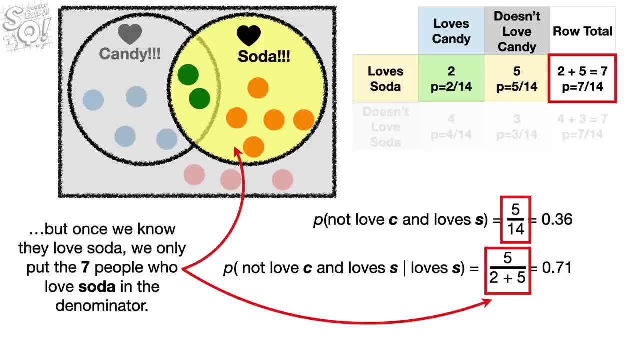 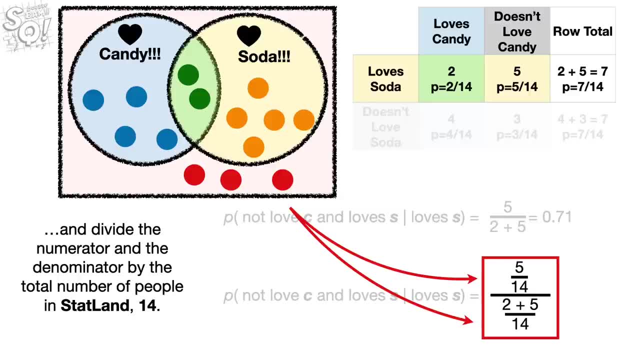 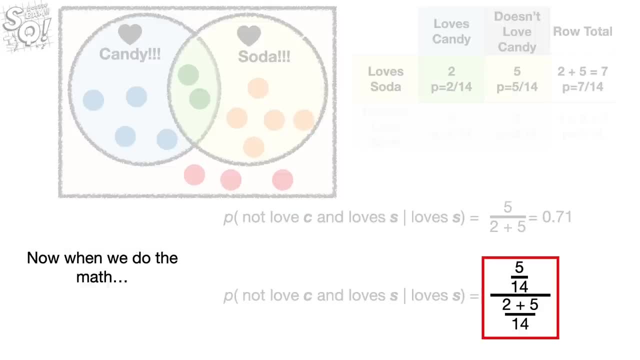 we only put the seven people who love soda in the denominator. Now let's make a copy of the conditional probability and divide the numerator and the denominator by the total number of people in StatLand 14.. Now when we do the math, we get 0.71,. 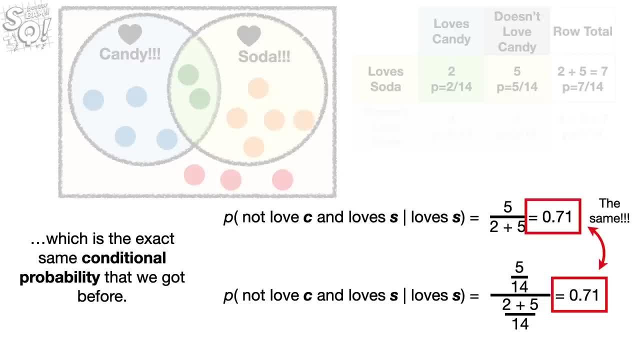 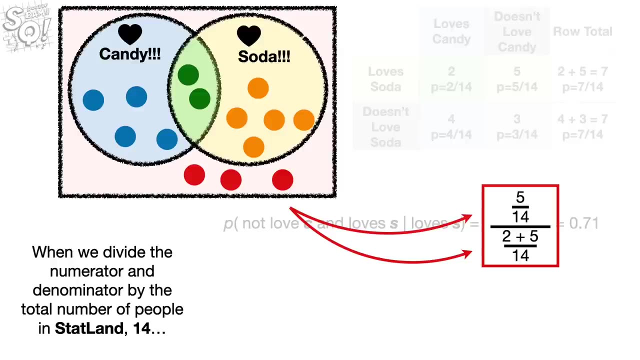 which is the exact same conditional probability that we got before. which is the exact same conditional probability that we got before. So what's the big deal about dividing everything by the total population? When we divide the numerator and the denominator by the total number of people in StatLand, 14,. 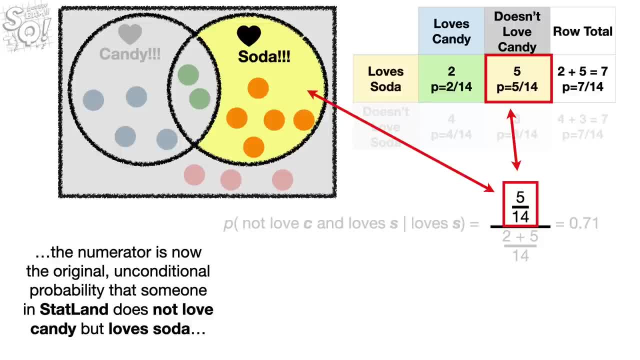 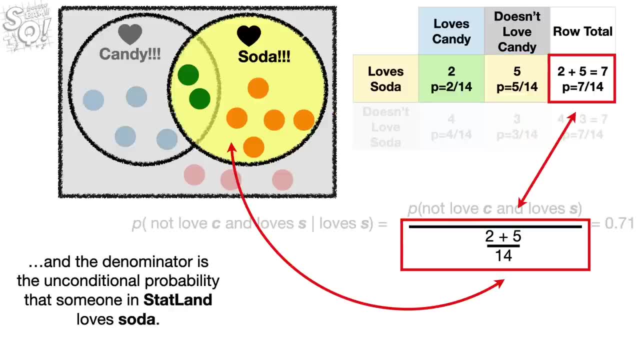 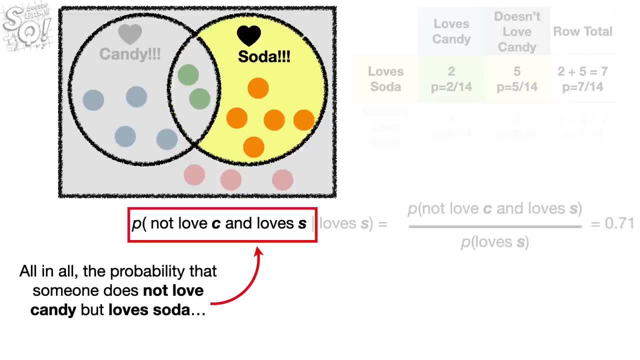 the numerator is now the original unconditional probability that someone in StatLand does not love candy but loves soda, And the denominator is the unconditional probability that someone in StatLand loves soda, and the denominator is the unconditional probability that someone in StatLand loves soda. 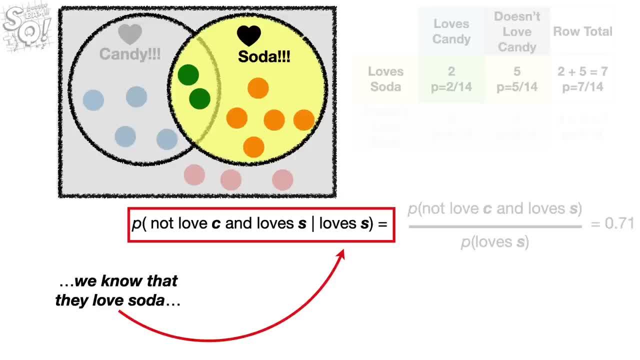 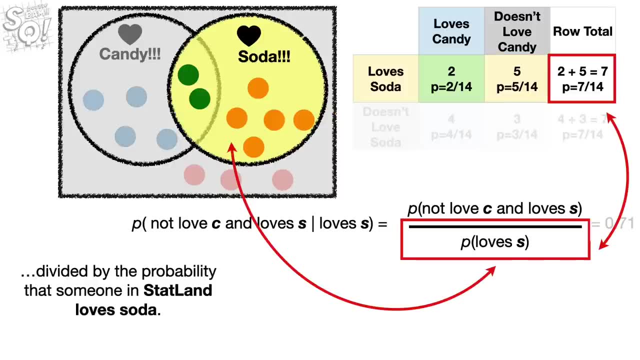 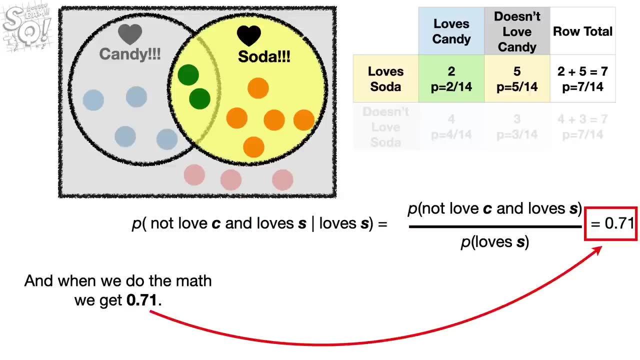 All in all, the probability that someone does not love candy but loves soda- given that we know that they love soda- is equal to the probability that someone does not love candy but loves soda divided by the probability that someone in StatLand loves soda. 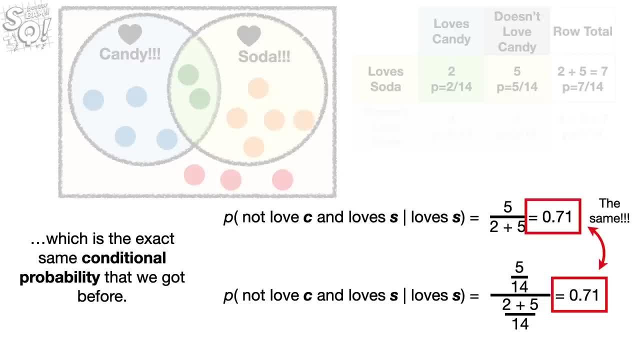 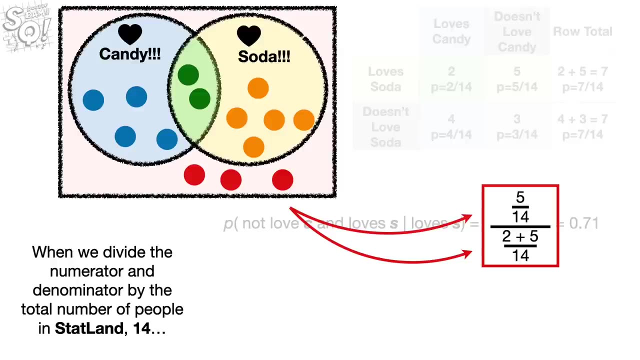 which is the exact same conditional probability that we got before. which is the exact same conditional probability that we got before. So what's the big deal about dividing everything by the total population? When we divide the numerator and the denominator by the total number of people in StatLand, 14,. 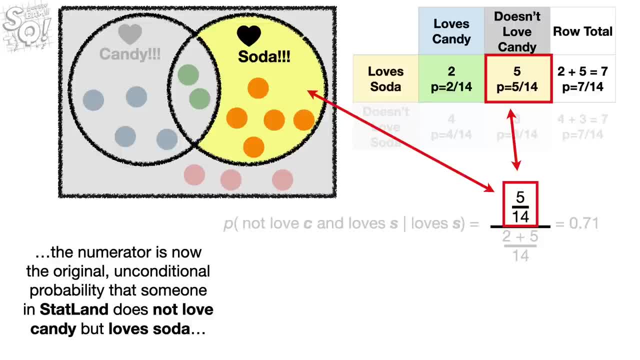 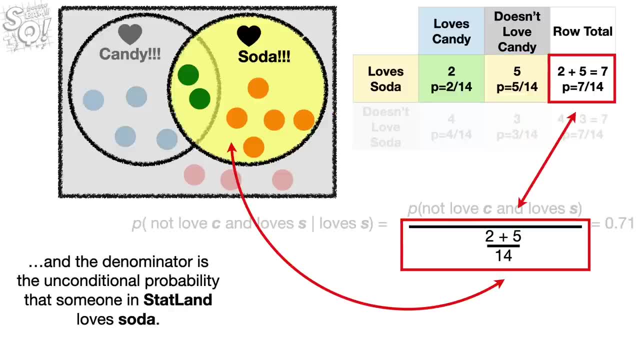 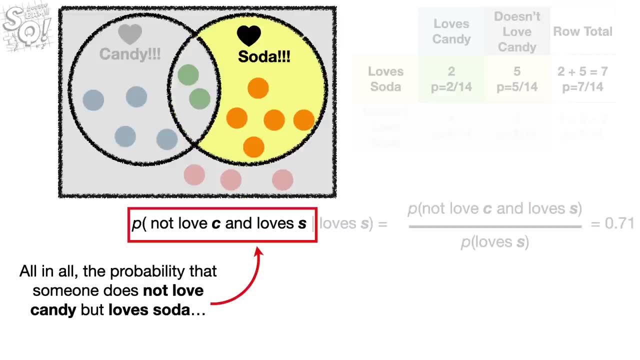 the numerator is now the original unconditional probability that someone in StatLand does not love candy but loves soda, And the denominator is the unconditional probability that someone in StatLand loves soda. All in all, the probability that someone does not love candy but loves soda, given that we know that they love soda. 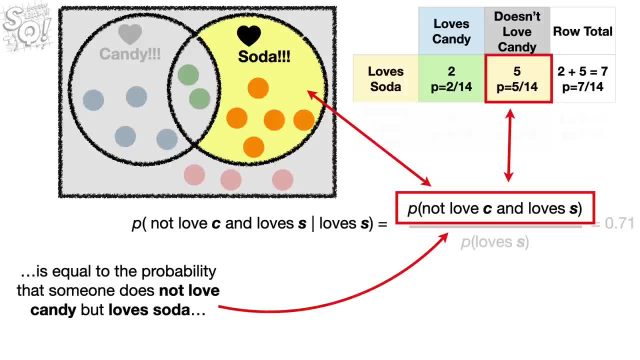 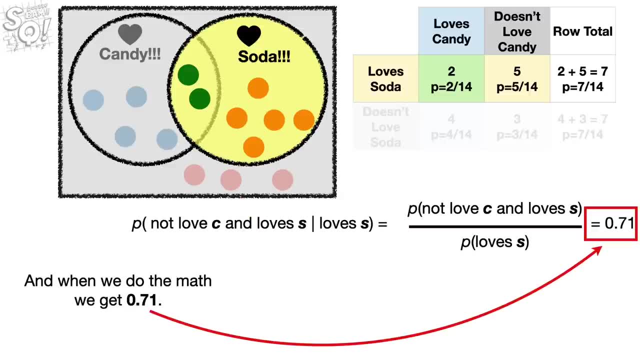 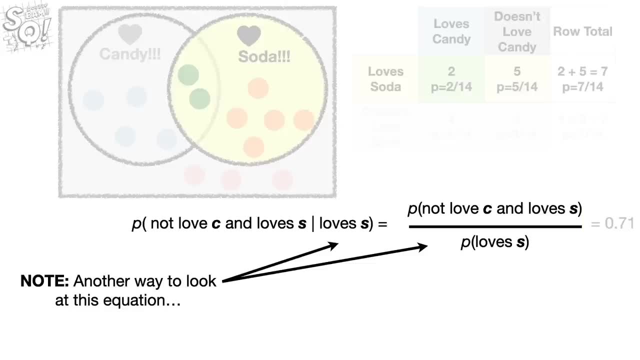 is equal to the probability that someone does not love candy but loves soda, divided by the probability that someone in StatLand loves soda, And when we do the math we get 0.71.. Note: another way to look at this equation is to realize: 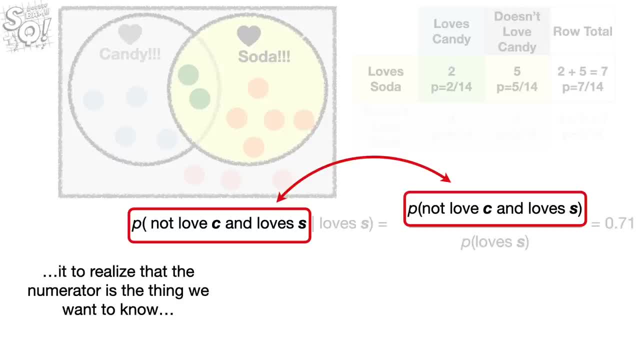 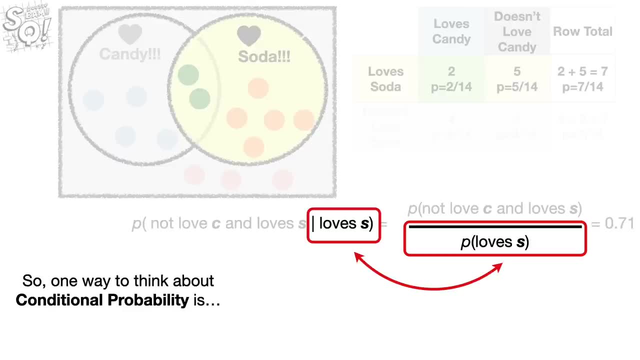 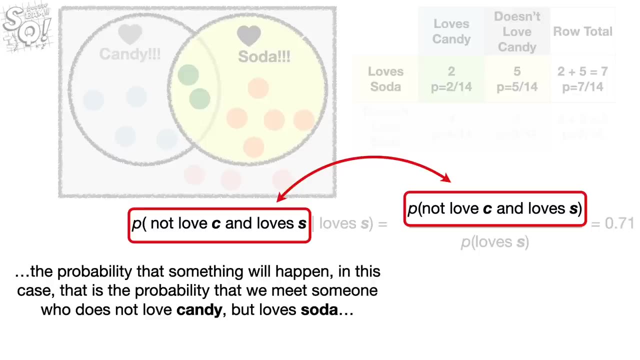 that the numerator is the thing we want to know and the denominator is the thing we know. So one way to think about conditional probability is the probability that something will happen. in this case, that is, the probability that we meet someone who does not love candy but loves soda. 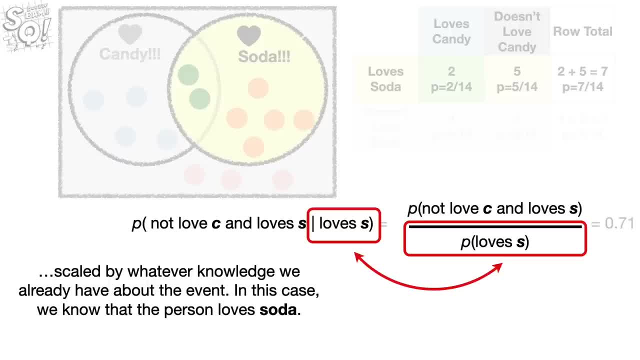 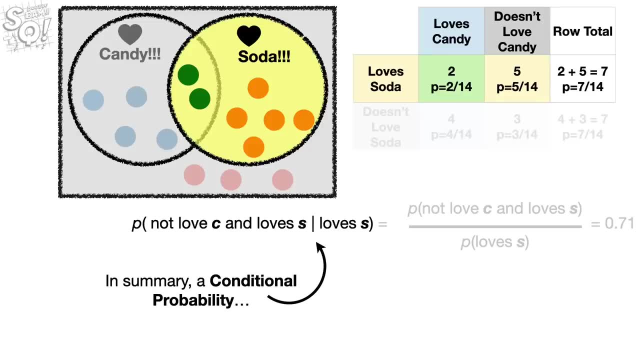 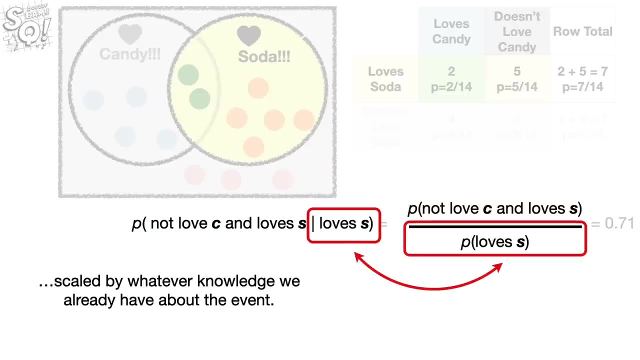 scaled by whatever knowledge we already have about the event. In this case, we know that the person loves soda and the denominator is the probability that someone does not love candy, And we can calculate the conditional probabilities with raw counts or the original unconditional probabilities. 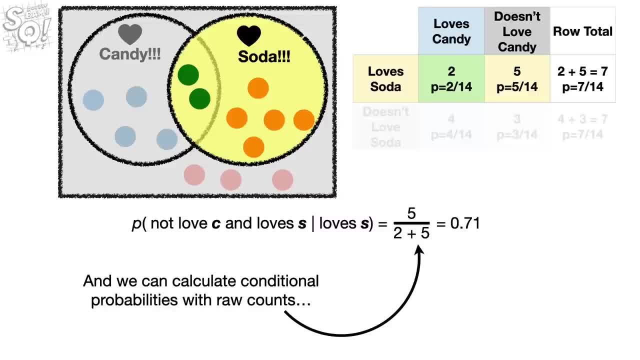 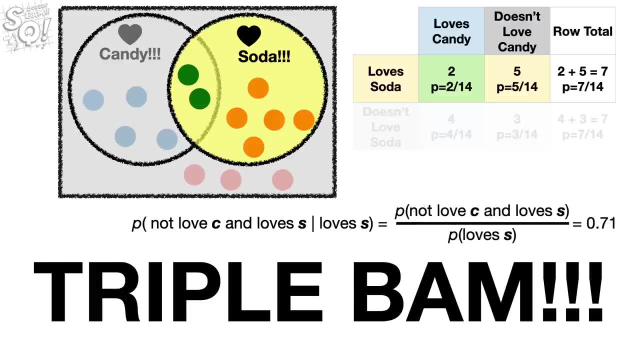 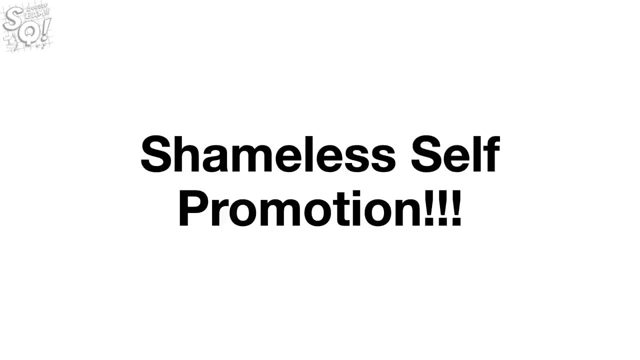 Triple bam. Now it's time for some shameless self-promotion. I'm going to show you how to calculate the conditional probabilities with raw counts or the original unconditional probabilities. I'm going to show you how to calculate the conditional probabilities with raw counts or the original unconditional probabilities. 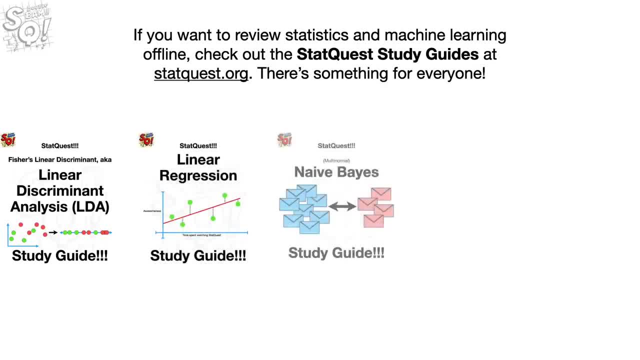 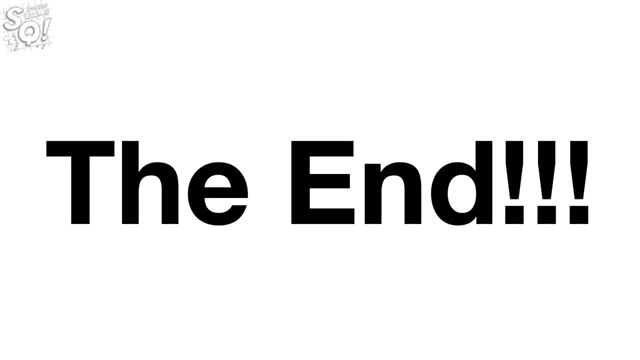 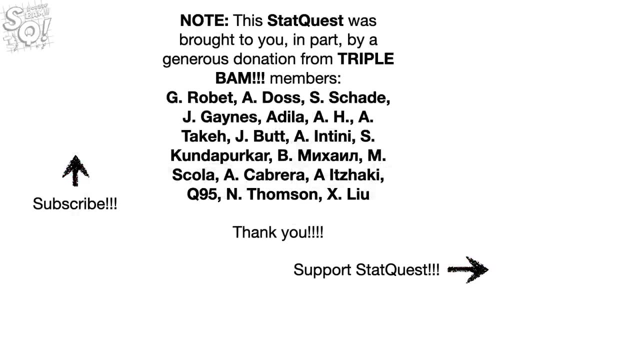 If you want to review statistics and machine learning offline, check out the StatQuest study guides at StatQuestorg. There's something for everyone. Hooray, We've made it to the end of another exciting StatQuest. If you like this StatQuest and want to see more, please subscribe. 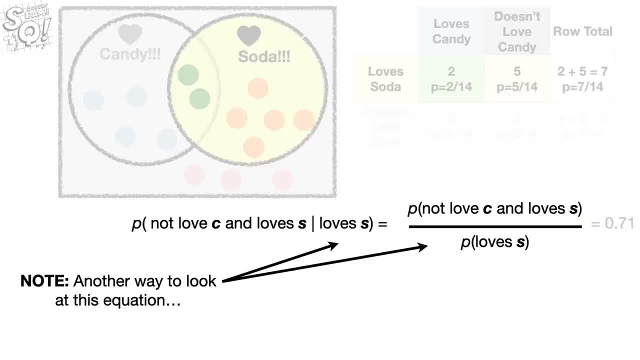 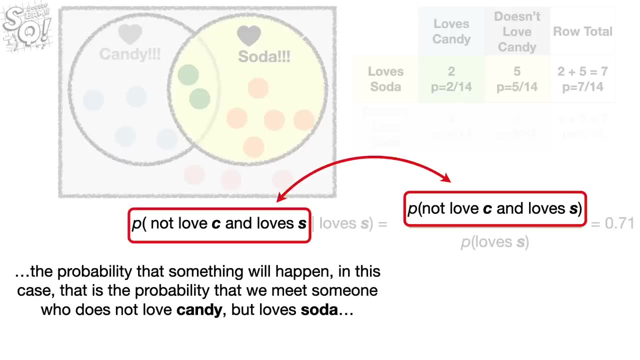 And when we do the math we get 0.71.. Note Another way to look at this equation: that the numerator is the thing we want to know and the denominator is the thing we know. So one way to think about conditional probability is the probability that something will happen.